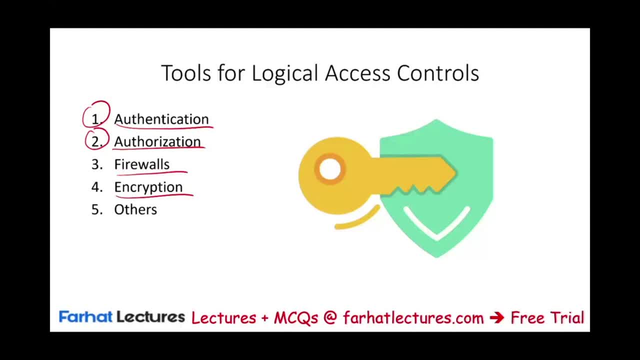 Many CPA candidates, many accounting students, don't know the difference between the two. So in this session we're going to go ahead and discuss both authentication and authorization. Let's go ahead and get started Before we proceed any further. I have a public announcement about my company. 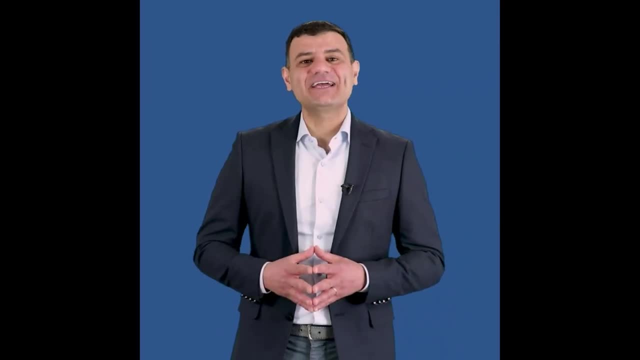 farhatlecturescom. Farhat Accounting Lectures is a supplemental educational tool that's going to help you with your CPA exam preparation, as well as your accounting courses. My CPA material is aligned with your CPA review course, such as the one I'm going to be talking about today. So if you 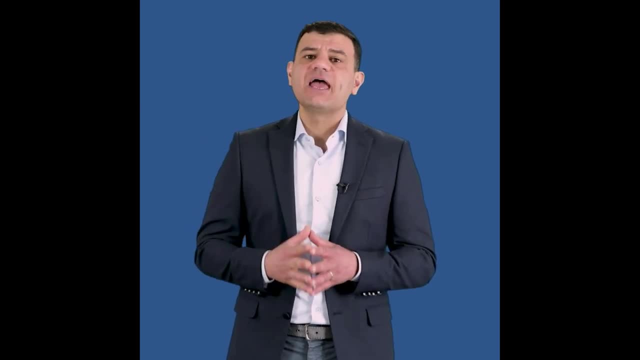 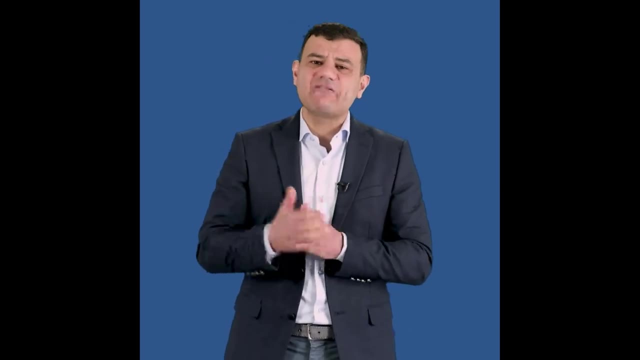 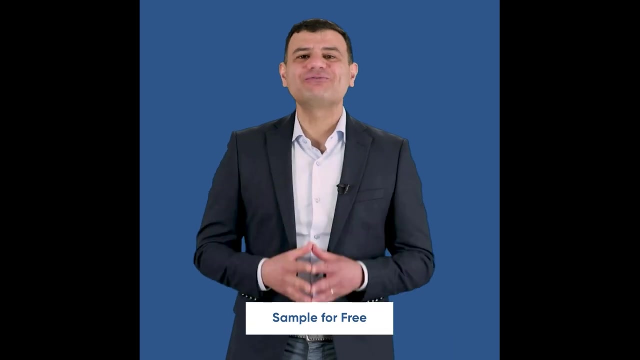 Roger Wiley, Gleam Miles. my accounting courses are aligned with your accounting courses, broken down by chapter and topics. My resources consist of lectures, multiple choice questions, true false questions, as well as exercises. Go ahead, start your free trial today. 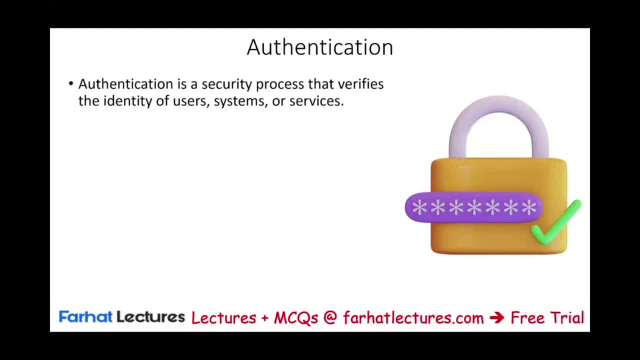 Authentication. What does it mean? It's a security process that verify, authenticate who you are, your identity, the identity of users, the identity of system or services It confirm: is it who you are? It's a fundamental component of logical access And 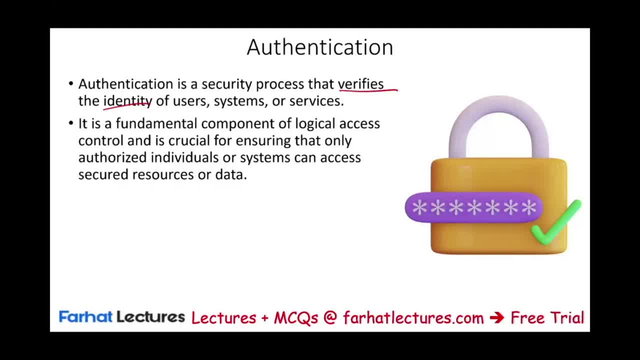 what are we talking about here? How do they make sure that's who you are? Think about password. That's the most simple logical explanation, But we have many type of authentication measure and this is what we will discuss here. So it's a fundamental component of logical access control. 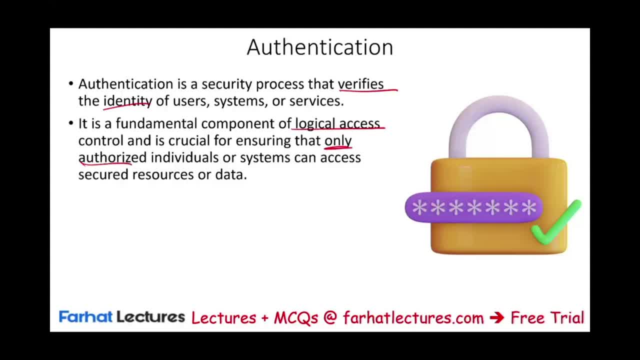 and it's a crucial for ensuring only authorized individual or system can access keyword resources or data. Now, how can we give this authentication? Well, sometimes it's something you know. Through that, something you know, something special you know. 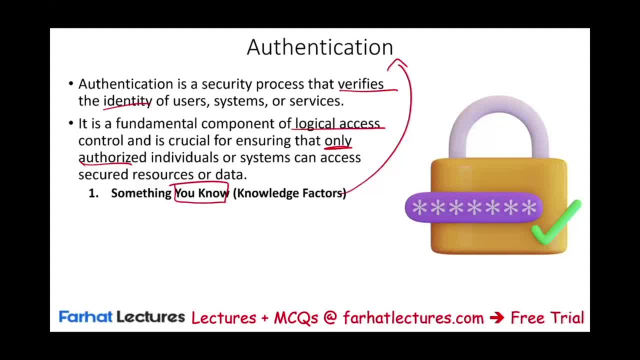 knowledge factor: we can authenticate you. For example, a password is the simplest example of this. We're answering a question, Something you have, something in your possession, in your hand. we're going to see what we mean by that Something you are. Inherence factor: We're. 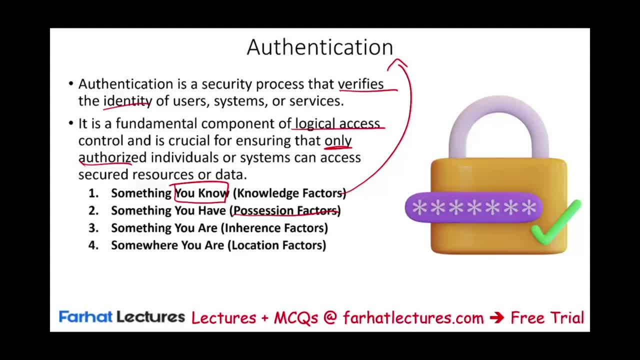 going to see what these are. Somewhere you are Could be a little bit Location factor That authenticate you Or something you do, Behavioral factors, And for each one of those we are going to discuss a little bit more in depth, starting with something. 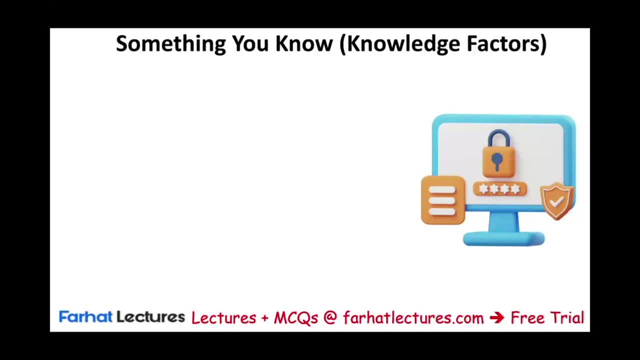 you know, Knowledge factor. The most common form of knowledge factor is, you guessed it- password, PIN, And we all should be familiar with passwords and PIN. If you're watching Farhat Lectures, you need it to access your account. You need to input your email and password. 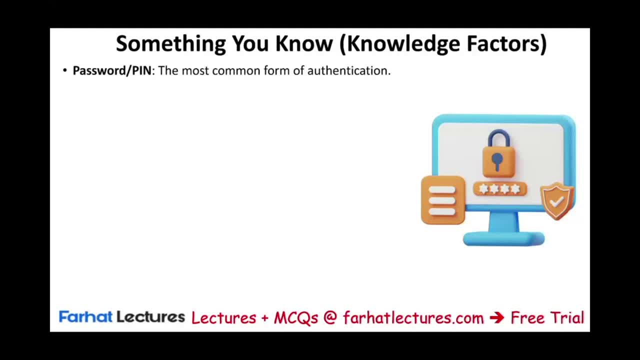 This is as simple as that. To log in on your computer or on your phone, you need to put a PIN or a password. Now it requires the user to provide a secret known only to them. This way, they can authenticate themselves to the system. Example: we'll be logging into an email account. 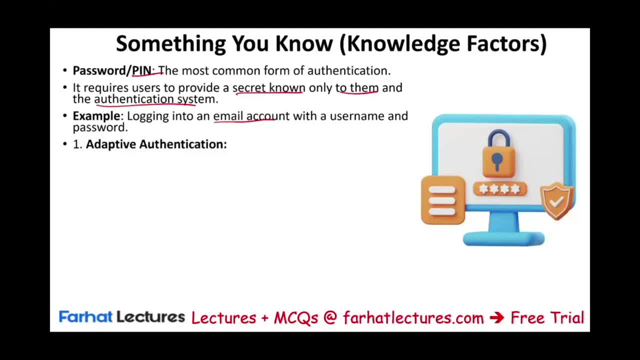 with a username and password. Now we have what's called adaptive authentication, So in addition to the password, we can use other attributes like device location, time of access, and we're going to look at all of those. For example, if you're not logging from a certain device, you are out. 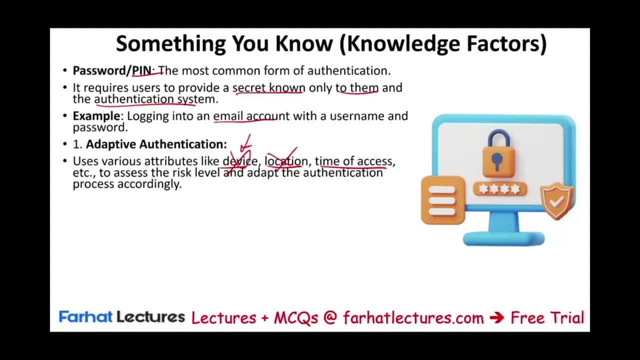 If you're not logging from a certain location, you are out. If you're not logging from it during a certain amount of time, you are out, And this is to assess the risk level and adapt the authentication process accordingly. To make sure who you are, we add other attributes and 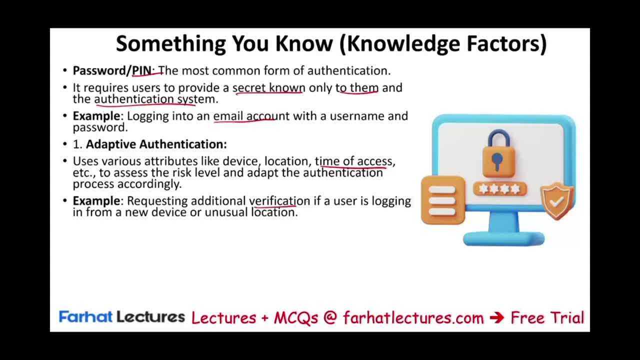 we're going to look at them. For example, we might request additional verification if the user is logged in in form of a new device or unusual location. For example, when I log in from another system, from another computer, to my work, at my work, it asks me to authenticate myself. It sends. 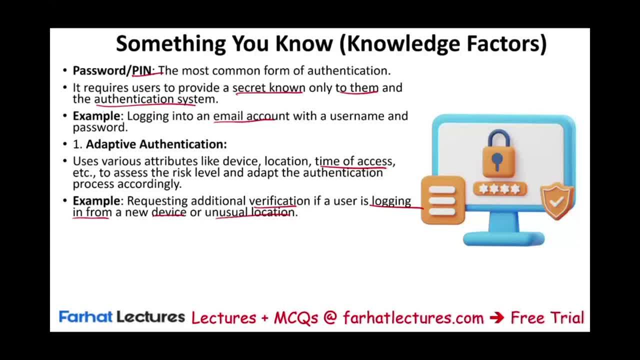 a message to my cell phone and I'll have to input this message. So, in addition to the password, the work system knows that I am logging in from an unusual place, not my usual place. That's why it will ask for verification. Sometimes you might have what's called single sign on or 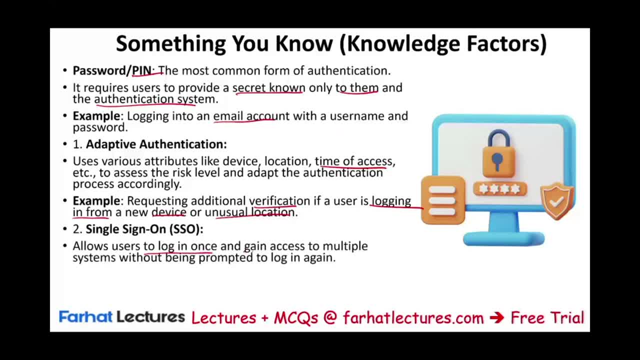 SSOs. It allows the user to log in once and gain access to multiple systems without being prompted to log in. A case in point here is we're talking about Google, When you log into your Google, Gmail, Google Photos, many Google services- without the need to log in separately. Now 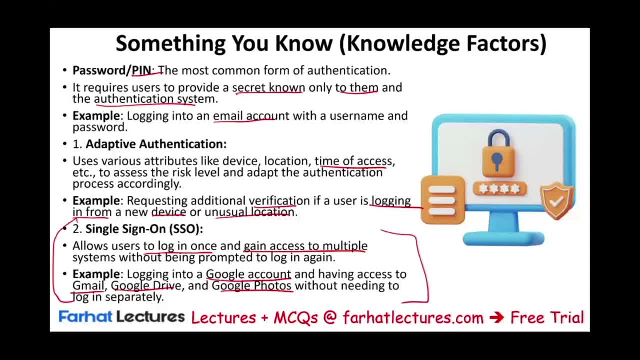 this is not really a it may not be the best secure system, but it's convenient, And if you trust Google, then you should be in good shape. But the password is something that you know. Something that you have is a little bit different. Here we're talking about security, talking or. 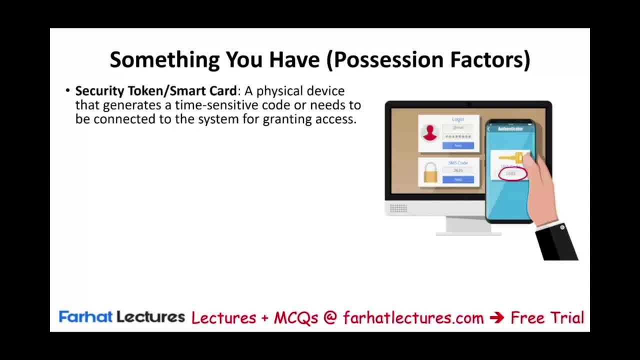 smart card or you would receive a code to your cell phone before you can access the information. So a physical device that generates a time-sensitive code or needs to be connected to the system for granting access. Now, tokens are basically a piece of hardware that generate numbers randomly every 30 seconds. So after you put 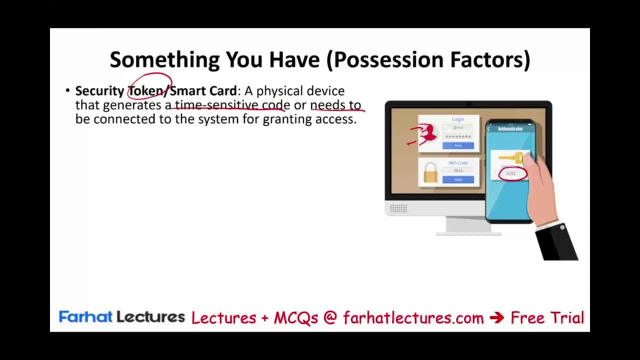 your login and password. after you put your login and password in banking system for certain accounts they have it. For example, I am, I'm still I am. I helped my brother with his own accounting, So I do have access to his banking account. So every time I log in I need that token. 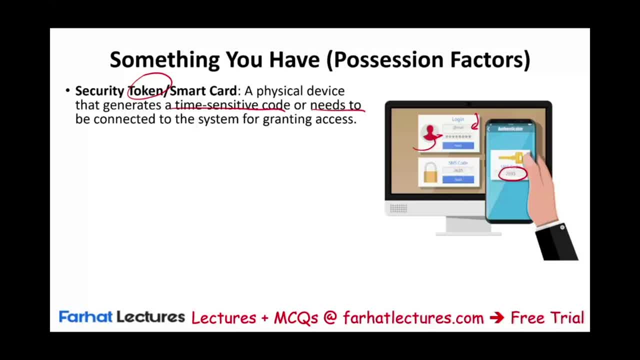 to generate a PIN number for me. So even if I lose my password, I'll need to lose the password plus the token in order to for the information to be compromised. So this is called the multi-factor authentication. So you are looking for more than. 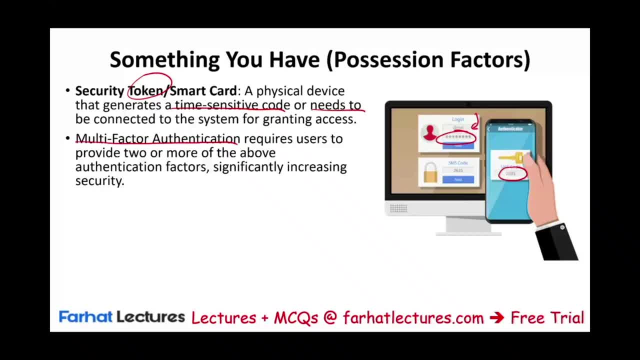 one thing: A password is good, but everyone thinks password is weak these days, So you need a password plus something else: sending you a message to your cell phone or having a security token. Sometime you might have a smart card to input in the system, So multi-factor authentication. 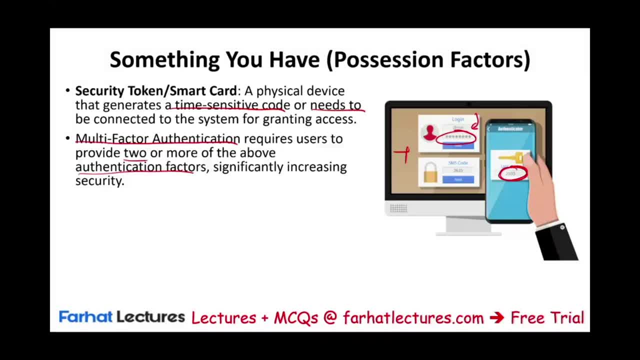 or more of the above authentication factor and, this way, increasing the security. Example: log in into a bank account online may require a password- something you know, that's fine- And a temporary code sent to your mobile device, and the picture here illustrate the concept. 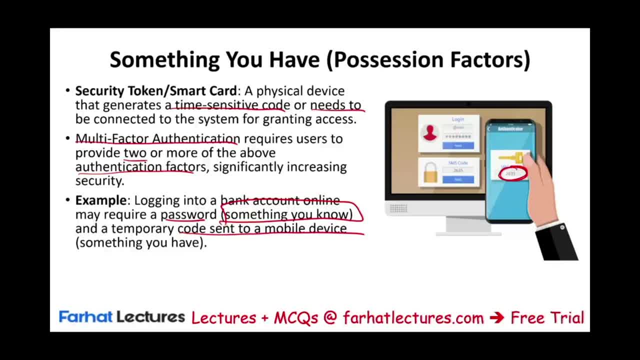 So, even if you lose your password, no one can log in unless they have your cell phone. example, using a hardware token, same thing that generate a temporary code to log into a secured system. Or you can have something you are inherence factor, which is, it's, very common. 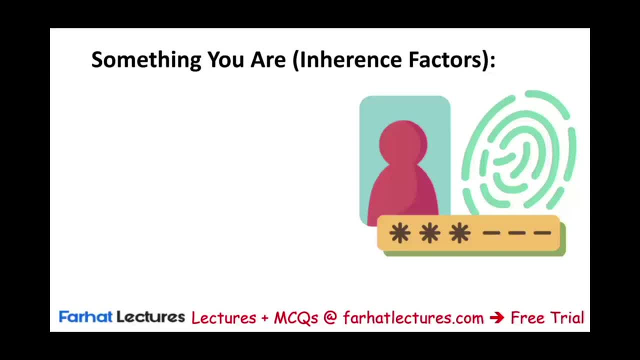 factor it's who you are, your, your biological footprint. basically biometrics, uses unique biological characteristic for identification. this examples will using fingerprint recognition or facial recognition or voice recognition. to simply put, for example, most phone: now they have facial recognition and with the phone, now they they can, they can also do facial recognition with. 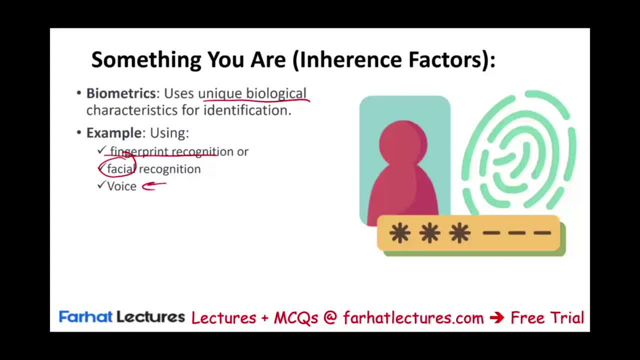 or without mask. this is post-covid. it's interesting voice. obviously, from your voice they know who you are. now, sometime when you call a customer service department, for example my brokerage account, they can verify me through my voice, for example, to unlock your phone. you could use the same type. 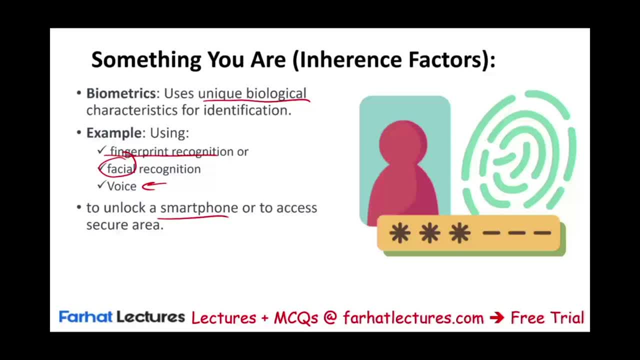 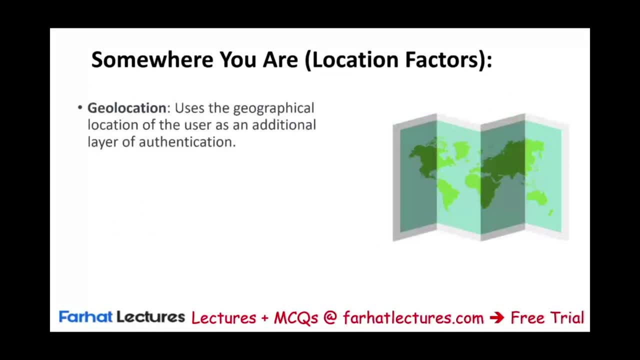 of technology or to access a certain area. if it's a secure area, sometime you are verified through a specific location location factor. geolocation uses the geographical location of the user as an additional layer of authentication. for example, you may not be able to access your business information or 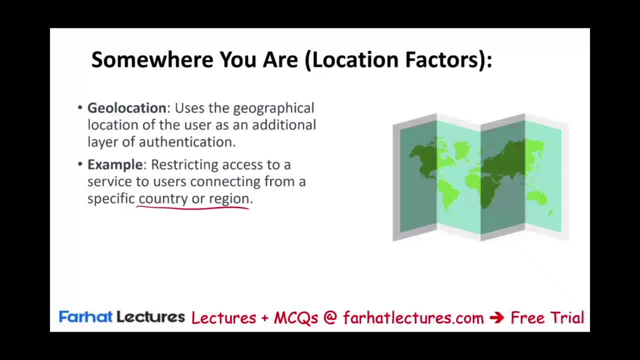 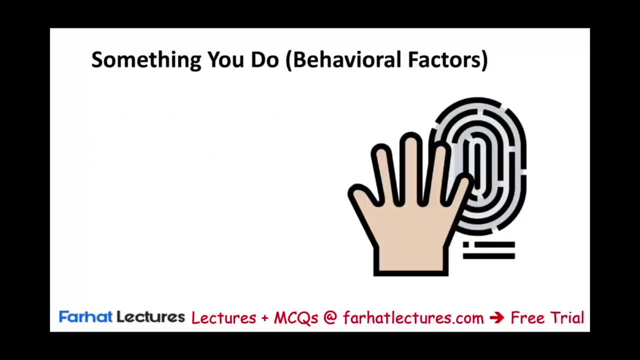 certain system, from a certain region or a country. so once you are there, that's it. they limit you, so you have to be someplace else. sometime. you can be authenticated through something you do, which is called behavioral factor. here you're analyzing the unique ways in which the individual interact. 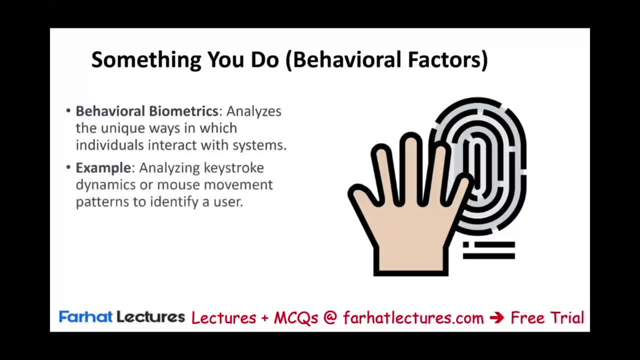 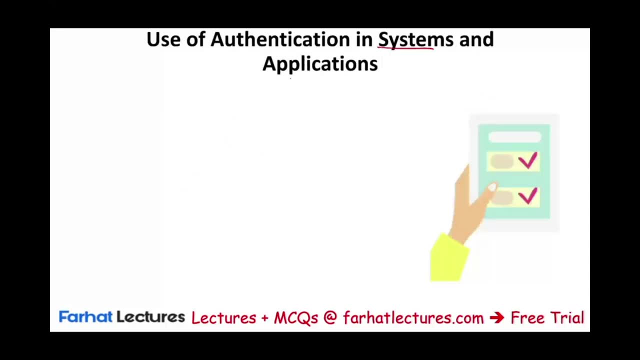 with the system. what are we talking about here is the keystrokes dynamics, how you type, or your mouse movement. each individual has a certain patterns and the system is smart enough to identify whether you are that user or not. also, we have authentication for systems and application those, if the other ones were specific. 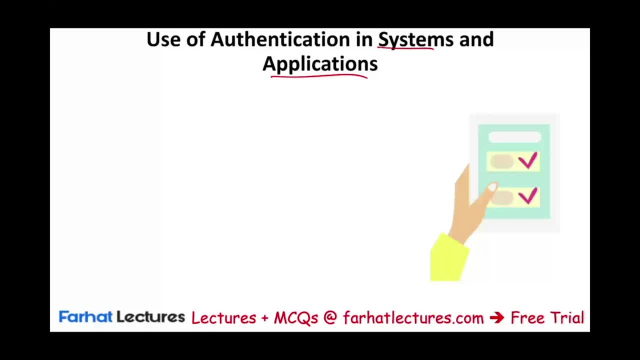 or application. these are general, not application specific. those are general. for example, almost every system and application require users act, user access, employ some form of verification, authentication. for example, if you log into your operating system, your windows, it requires you to log in with a username and password and possibly a second factor like a fingerprint. most web 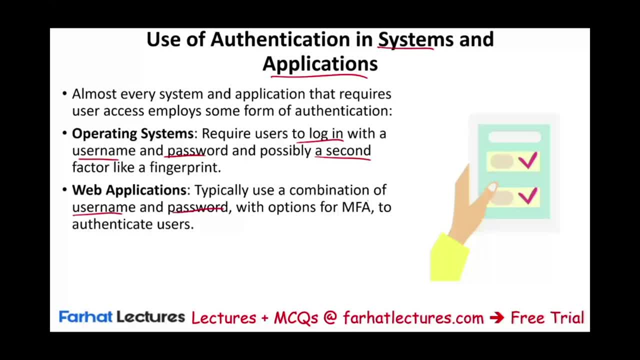 application typically use a combination of username, password with options for mfa multi-factor authentication to make sure that's who you are. mobile apps: many mobile app use biometrics like facial recognition fingerprint. we talked about this in addition to or instead of the password. so notice: password. it's not going away, but password can be easily- easily- not easily, but it. 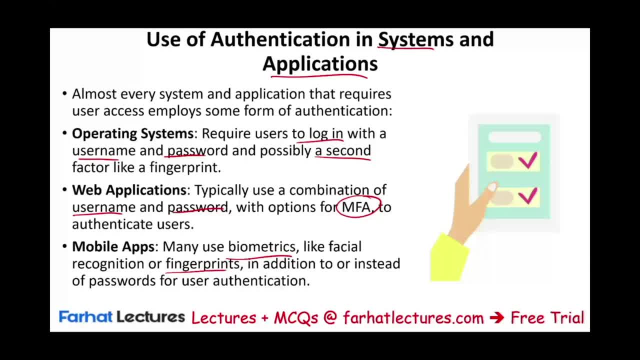 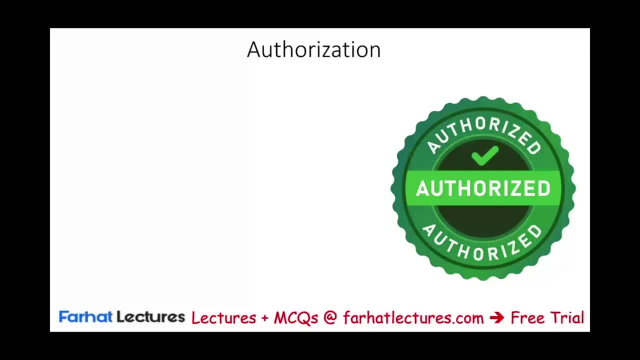 can be guessed, so we need multi-factor authentication. that's kind of what's going to increase the security. now we're going to move from authentication to authorization. some people think they're the same. they're not the same. we need to understand the difference between the two. authorization is the process that comes after. 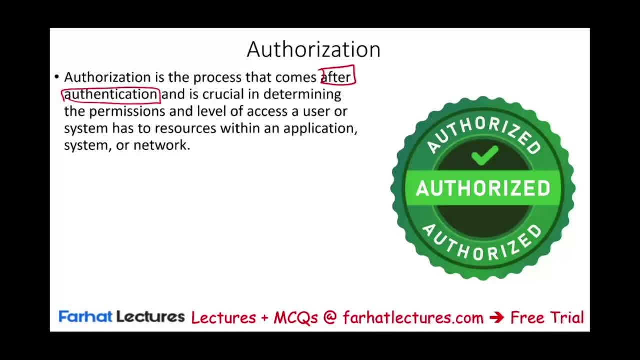 after you've been authenticated. now we're going to tell you what you can access or not, and it's crucial in determining the permission and level of access. a user or a system has two resources within the application system or Network. so, after you're logged in, what do you have access? 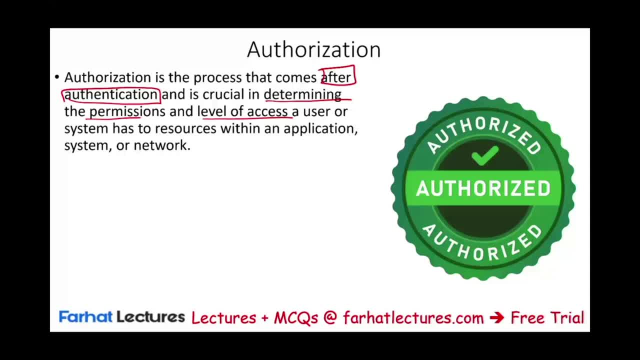 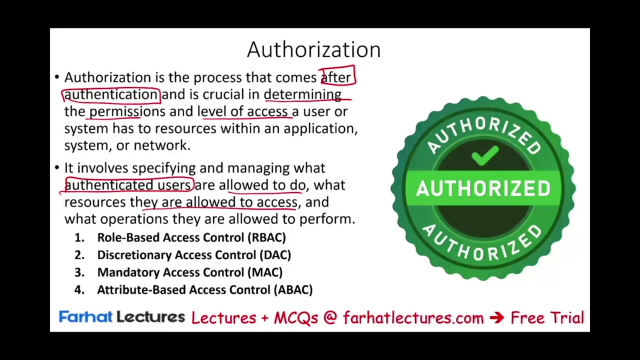 to that matters. there are different level of authorization. different level of authorization Here we involve specifically identifying and managing what authenticated users- already has been authenticated- are allowed to do, what resources they are allowed to access and what operation they are allowed to perform. There are a few of them. We have role-based access control- RBAC- We have discretionary access control- DAC- We have mandatory access control- MAC, And we have attribute-based access control- ABAC. Obviously, we're going to go through each one, making sure we understand it. 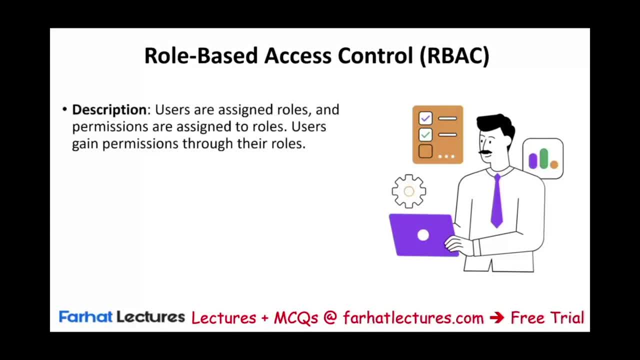 Role-based access control. Basically, the users are assigned roles and permission to whatever roles they play. Users gain permission through the roles, whatever the role is A user assigned. the role of manager may have read-write access to certain file, while a user with the role of employee may only have read-only access. 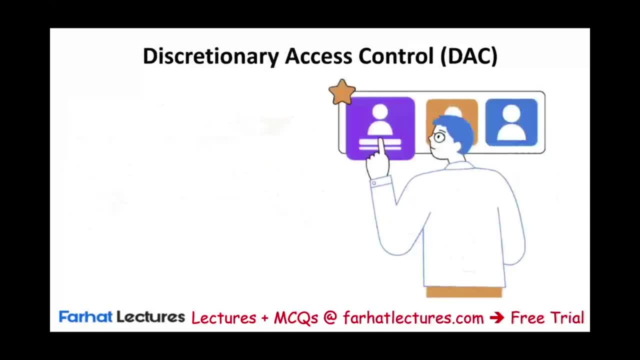 So, based on your role, you have the access. We might have discretionary access control. Owners of the resource have discretion over who has access and what kind of access. What are we looking at here? A user can create a file and grant read-or-write access to other specific users, So they have discretionary. They can give it, take it away. Usually those are admin people. 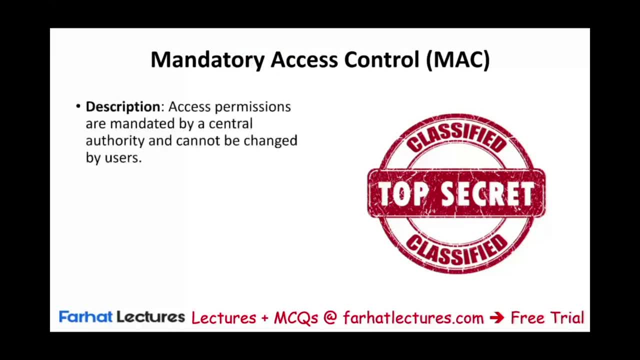 Mandatory access control Here. what we're talking about is permission are mandated by a central authority and cannot be changed by user. For example, when the government have top-secret information, you cannot access it if you don't have the clearance level. That's it. 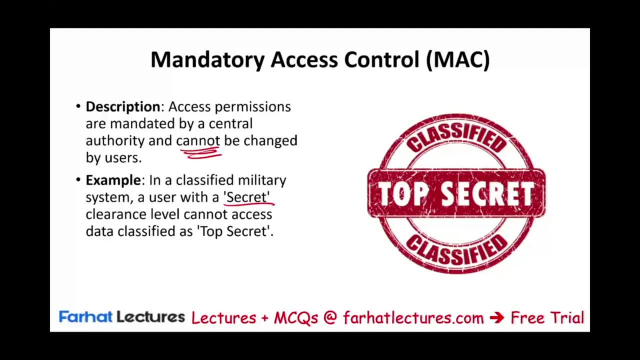 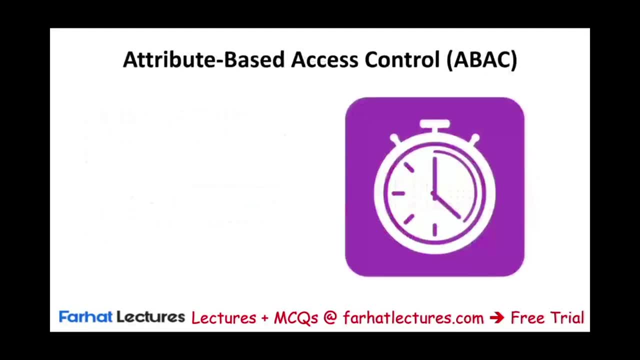 Classified military system. a user with a secret clearance level cannot access top-secret. It does not matter, It does not allow it. That's it. You are prohibited. You could have attribute-based access controls- ABAC. Here you're using attributes like what Your department based on your department or location or time assigned to users and resources to determine access. 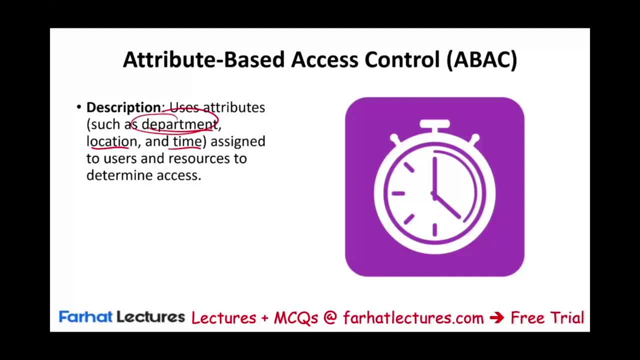 So if you work in that department, you have certain privilege and certain access, or in a certain location or time. What do we mean by time? For example, a user from the HR department may only access employee record during office hours, but it's restricted after office hours. So we don't want you to be able to access this information when you're not supposed to. 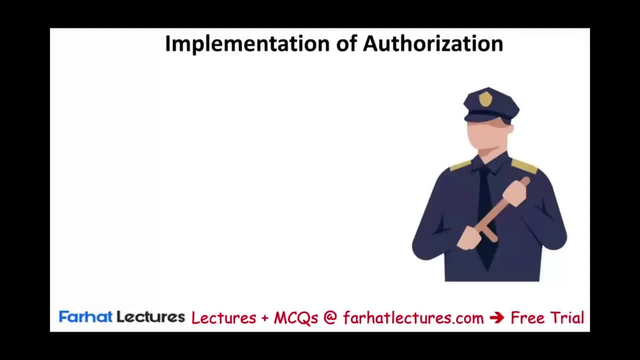 Implementation of authorization. How do we make sure that authorization is being followed? One thing we could have is policy enforcement: Define and enforce what resource users can or cannot access. How do you enforce this? really, Create a firewall Blocking traffic based on certain rules. You could have constraints. Those are additional restriction or condition applied to access. 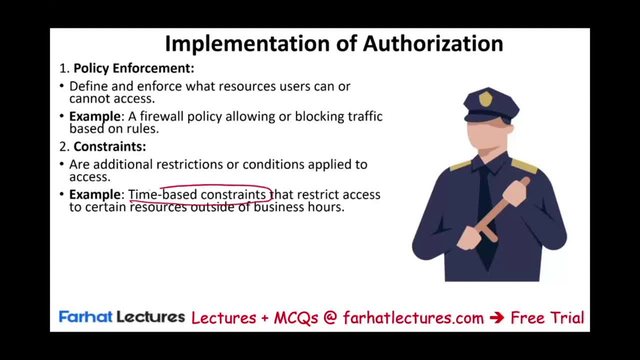 So, if you want to, for example, time-based constraint, this is a constraint that restricts access to certain resources outside of the business hours. So you add more constraint in addition to the authentication, In addition to the authorization, you might have other constraints. 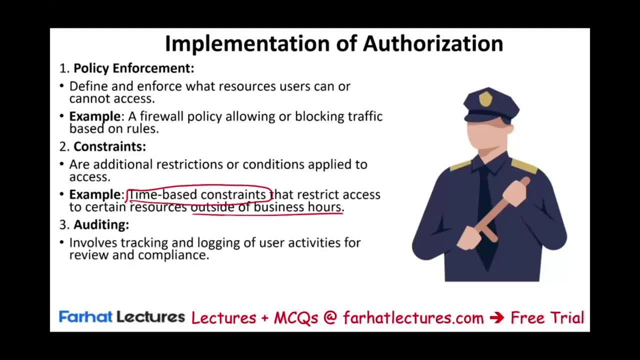 Auditing. Basically what's auditing? Reviewing what's going on, Involving tracking and login of user activities for review and compliance. A log showing who accesses a specific file and when You want to know what's going on. This is how you make sure the authorization is being followed properly. 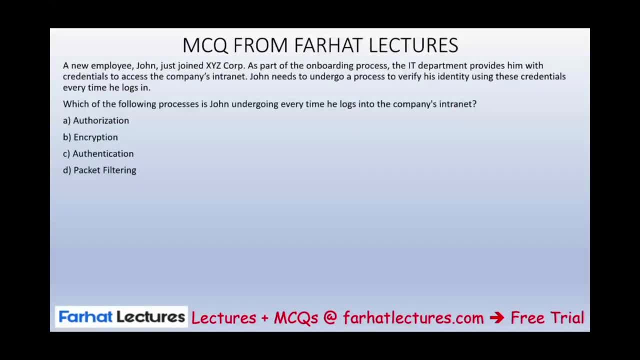 Let's take a look at a multiple choice question from Farhat Lectures that's going to help you understand this topic better. The question reads: which of the following process is John undergoing every time he logs into the company Intranet? Okay, A new employee. John has just joined XYZ Corporation. 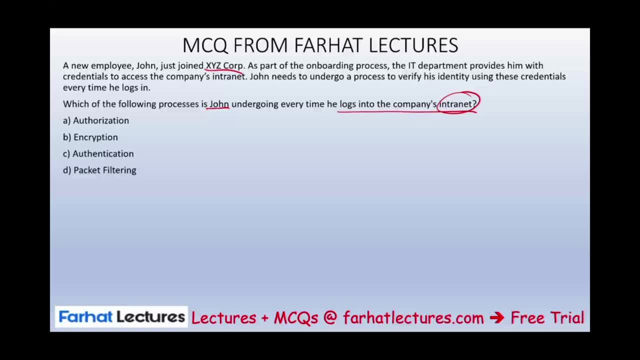 Part of the onboarding process, the IT department provide him with credential to access the company Intranet. That's what they provided him. John needs to undergo a process to verify his identity using these credentials every time he logs in. So what are we talking about here? Is it authorization, encryption, authentication, packet filtering? Which one is this? 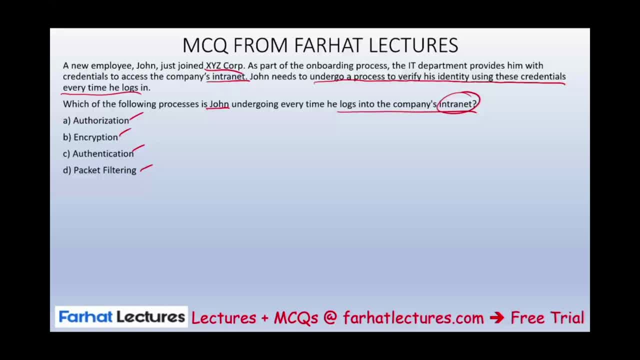 Well, let's kind of eliminate the options that we did not cover in this session. We did not cover encryption, But again in the real world, Not in the real world On the exam, on the CPA exam. you cannot say we did not cover this.